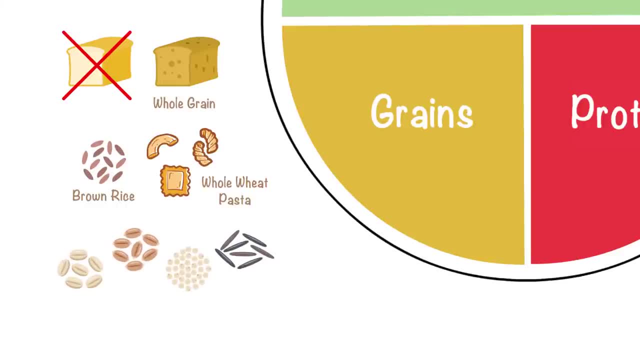 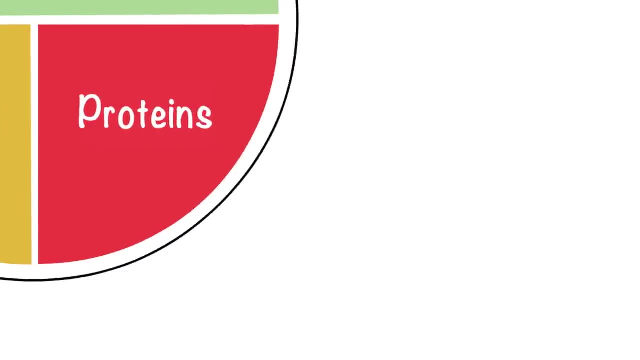 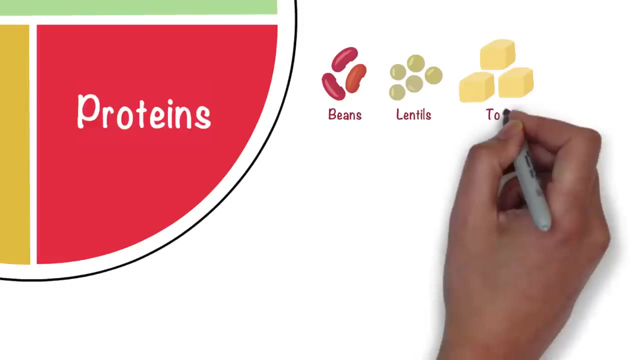 when preparing meals. Try different grain products such as pot, barley, bulgur, wheat, quinoa and wild rice. Eat more plant-based sources of protein, such as beans, lentils and tofu. Try to eat at least two servings of fish per week. 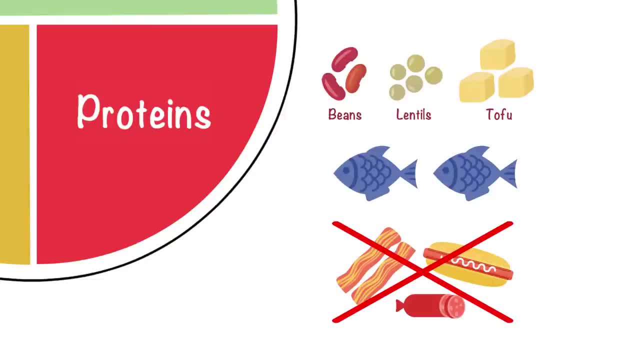 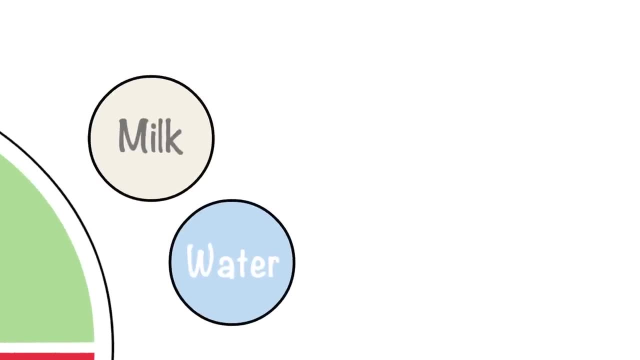 And limit deli meats that contain high amounts of sodium or salt, such as bacon, ham, hot dogs, pepperoni and salami. Serving two cups of milk every day can help your child's bone development If choosing alternatives like soy or almond milk. 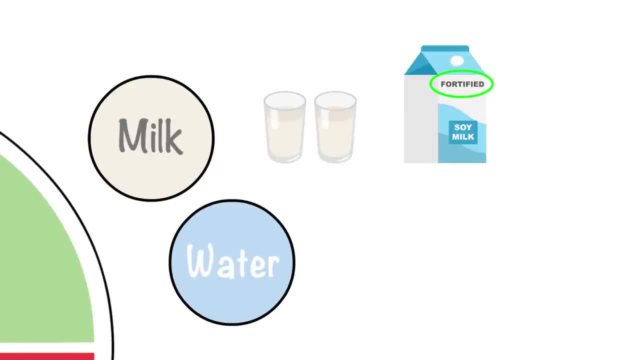 make sure they're fortified. This means nutrients like calcium or vitamin D have been added. Avoid sugar-sweetened drinks such as pop and fruit drinks. They have a lot of protein, They have a lot of calories, but contain few or no nutrients. 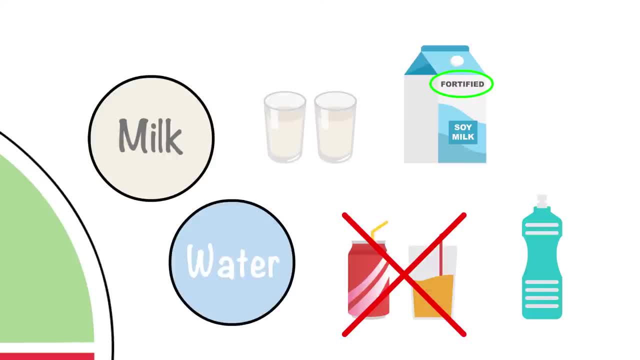 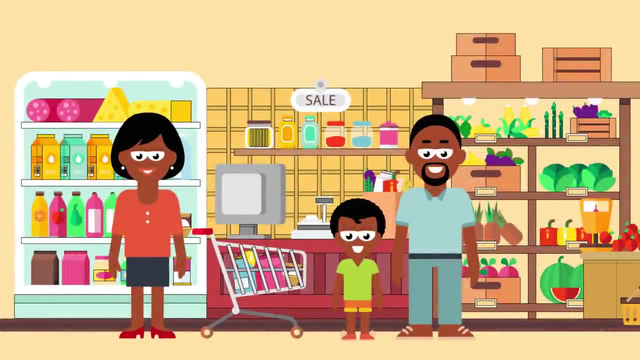 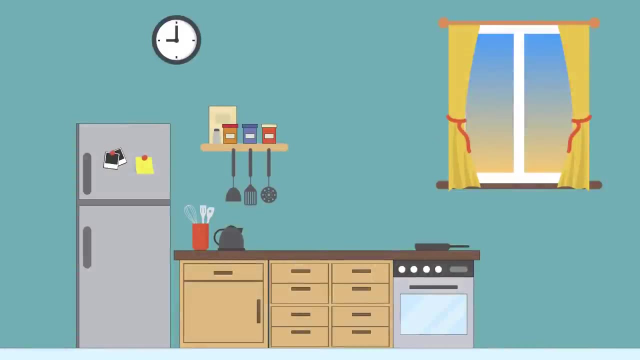 Encourage your child to drink water and pack a reusable water bottle for school and other outings. Remember all these tips when you're shopping at the grocery store. Good choices start there, Now that you know what foods your child should be eating and how to select the best options. 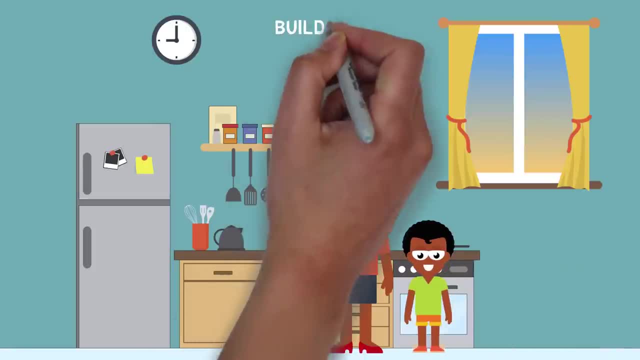 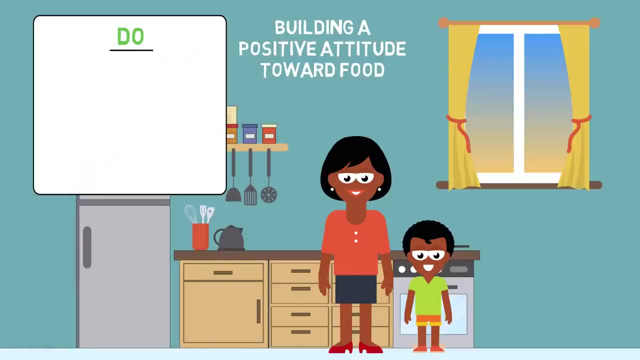 how do you get your child on board? Follow these tips with your child to build a positive attitude toward food. Here is a list of do's. Prepare meals with your child. They are more likely to eat food if they're involved in making it. 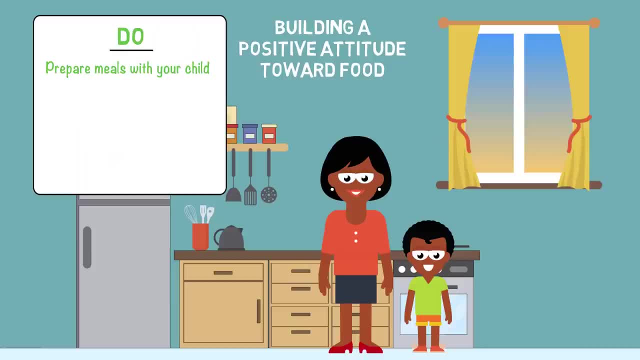 Experiment with new foods And remember it can take several tries before your child enjoys eating something new. Lead by example. Your child is more likely to try new foods if you eat them too. Turn off the TV and put on a mask. 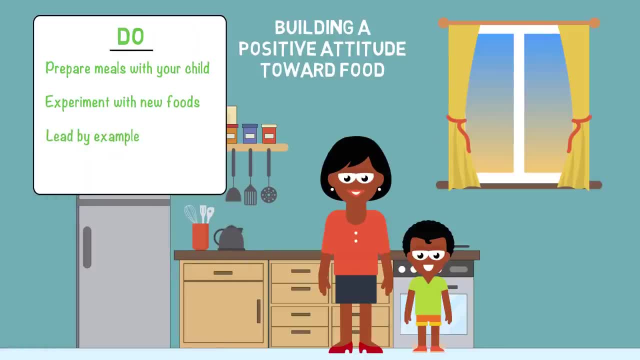 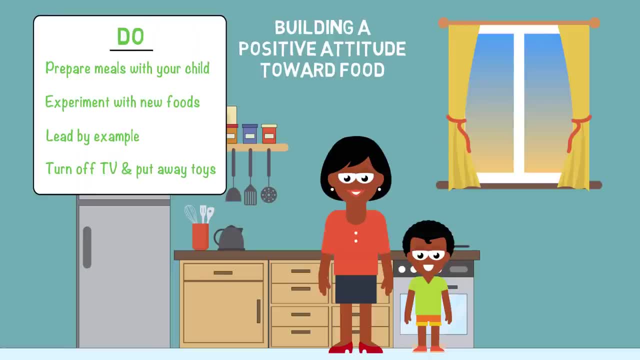 you can put on a face mask. Don't eat and put away toys during mealtime. Children eat better without these distractions. Children eat better without these distractions. Here is a list of don'ts. Here is a list of don'ts. 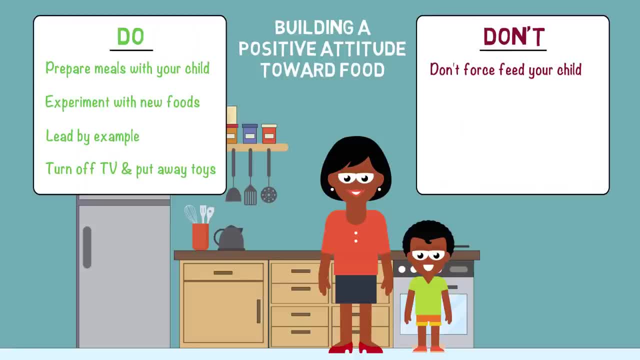 Don't force feed your child. Let them decide how much they want to eat. Let them decide how much they want to eat. Avoid skipping meals. Make it a routine and offer your kids healthy meals and snacks. Make it a routine and offer your kids healthy meals and snacks.